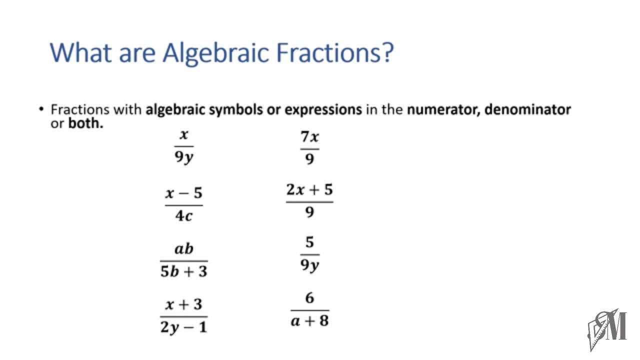 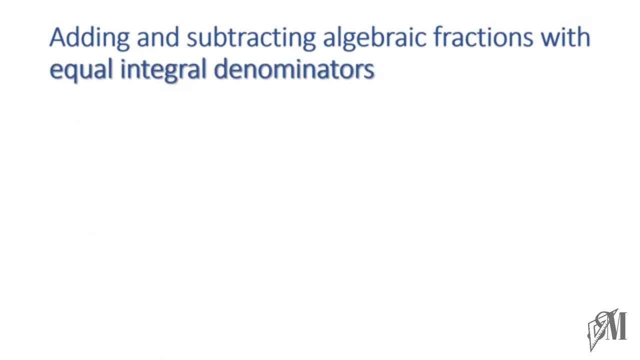 Let us move on. The first part we are going to see is adding and subtracting Algebraic Fractions with equal integral denominators. Here, integral denominators means the denominators will be numbers. Now look at this example: 7x over 9 and x over 9.. The denominator in both the fractions 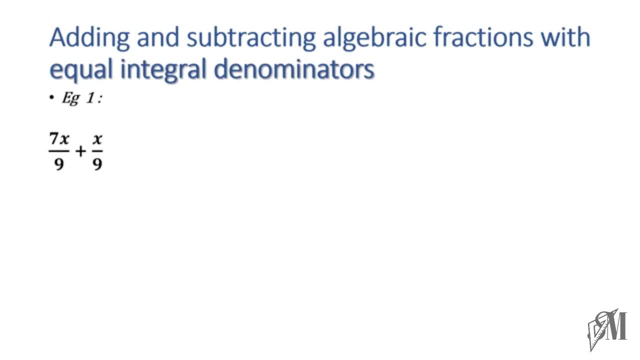 are 9.. So this is a very simple addition. What you have to do is just add the numerators, because the denominators are same. Now what we do is 7x plus x over 9, that is, 8x over 9.. Moving on to the second example, Here there are 3 fractions: Addition and 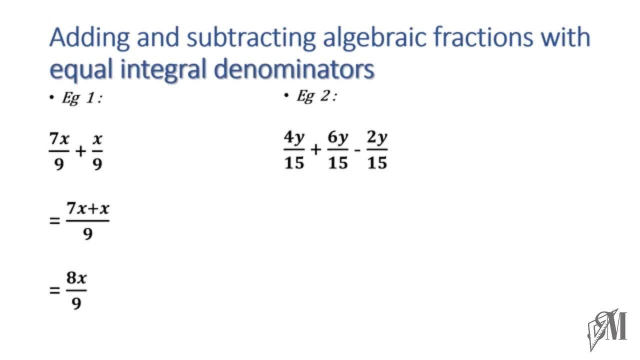 subtraction is available: 15 is a common denominator for all the 3 fractions. So we can write 15 as the common denominator and write the rest in one line: 4y plus 6y is 10y is 8y over 15.. Moving on to the third example: t plus 1 over 4 plus t plus 5 over 4.. Now, 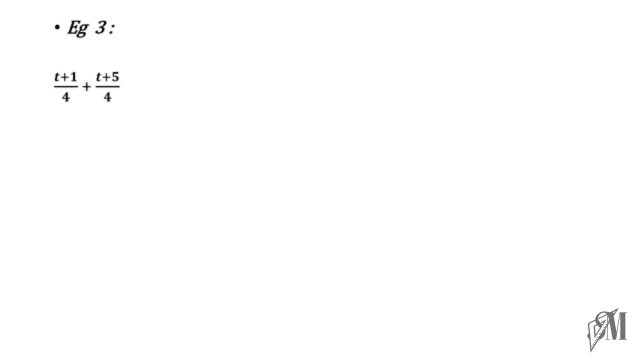 here. this is somewhat different from the previous two examples, because in this case the numerator is an Algebraic expression. So here, since it is addition with the same denominator, we write everything together like this: Now you can see t plus 1,. 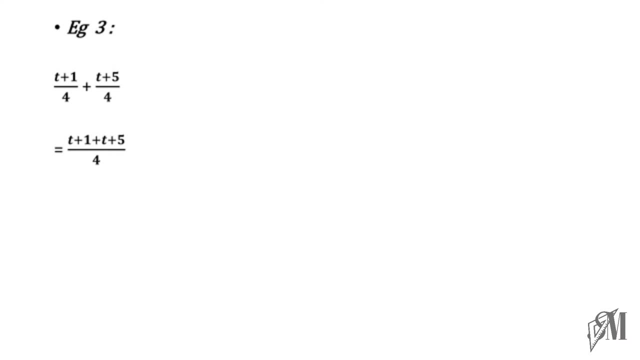 plus t plus 5.. You know, t plus t is 2t, 1 plus 5 is 6.. So you can write 2t plus 6 over 4.. The final example under this topic Now, in this case, once again the denominator. 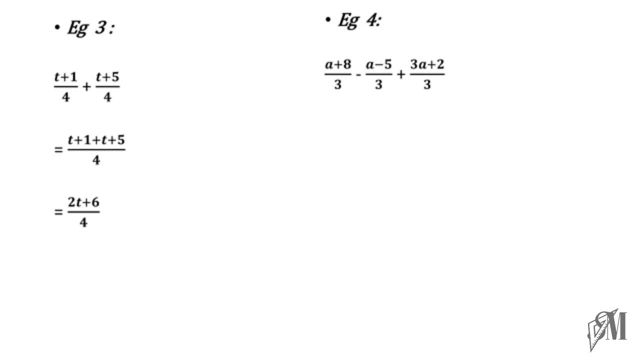 is 3, and here you have subtraction as well. Remember, children, when a subtraction comes Among the fractions, you have to take care to write the expression after the subtraction sign within brackets like this. Now, here you can see, I have written a plus, 8 minus since it is coming. 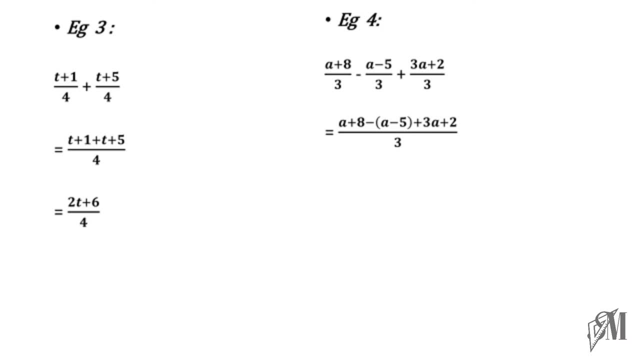 after a minus, the next part I have put within brackets and then addition sign. no problem, you can write as it is, but when subtraction comes- this is a very important place where you do mistakes- definitely you have to write the expression within brackets and then in the next step we 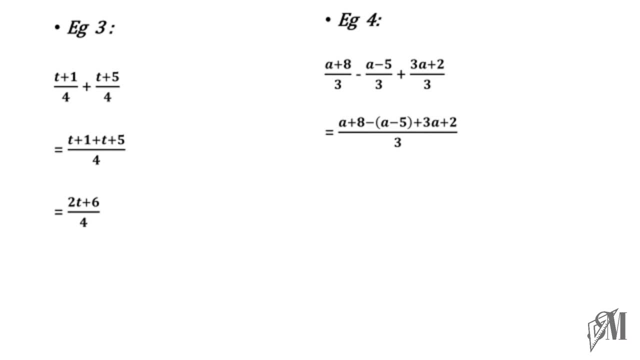 have to remove the brackets. that is, we multiply each term inside the bracket by minus sign, like this. Now, here you see, this minus into a is minus a and this minus into minus 5 is plus 5. so likewise, it is very important, that is what I am telling you. 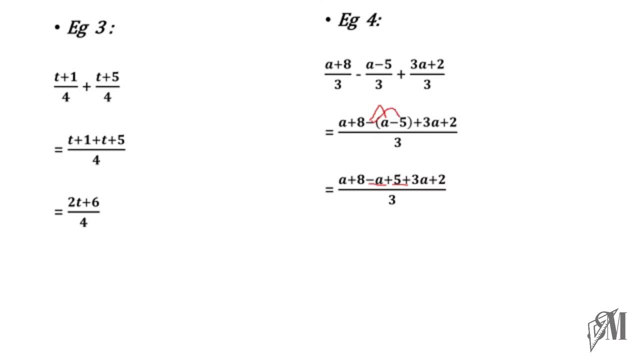 To make sure that you write within brackets the expression which is after minus sign and then this hereafter. it is simple, just usual simplification: a and minus a. Now, in this case, this plus a and minus a can be cancelled: 8 plus 5 plus 2 will be. 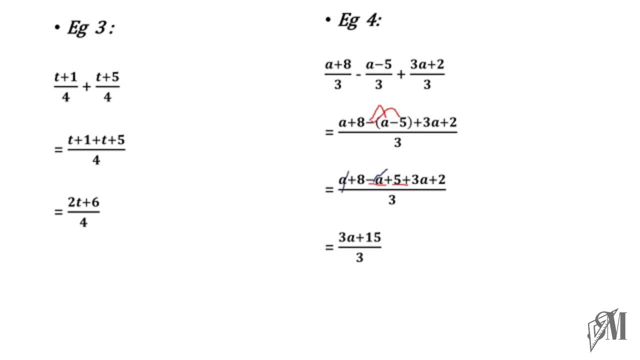 15 and that 3a we write as it is 3a plus 15.. Now in this case you can see you have already learnt factorizing. so 3a plus 15 can be factorized. both 3 and 15 are multiples of 3. therefore you can take 3 out of a bracket. then you get it like this: 3a plus 5. 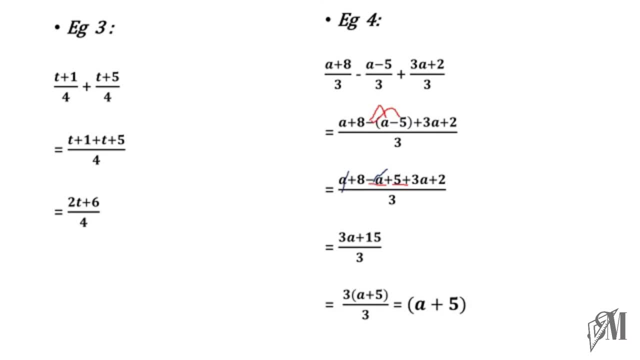 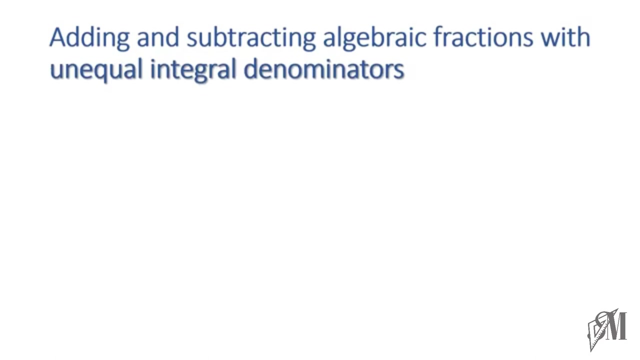 over 3.. Now here, what I have done is this: 3 can be cancelled with this 3, so the answer is a plus 5. right Now let's move on to the next part of this Topic, that is, addition and subtraction of algebraic fractions with unequal integral. 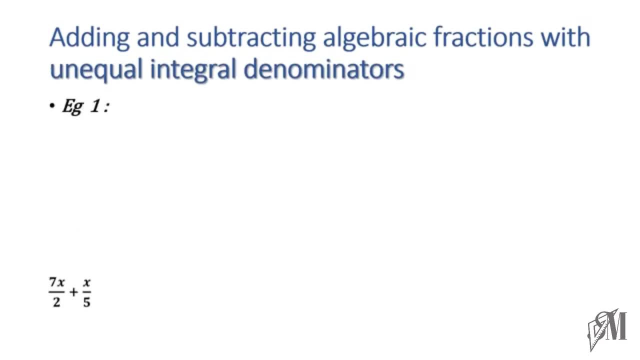 denominators. Now, when it comes to an unequal integral denominator like this, normally in simple simplification of fractions, you know if the denominators are not equal, in order to add or subtract you have to equate the denominators. So 2 and 5, the least common multiple of 2 and 5. 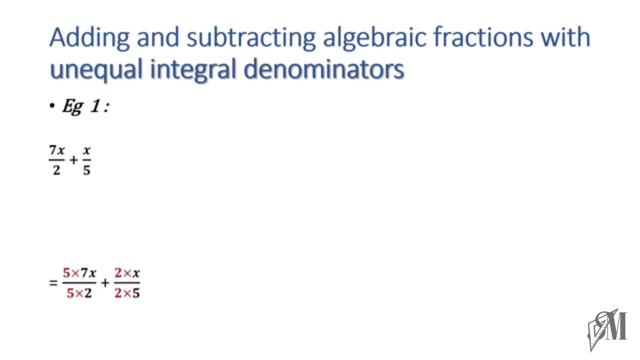 is 10. so we equate both to 10. like this: The first fraction we multiply by 5, the second fraction we multiply by 2.. This is a very simple case. Then you get the common denominator as 10 and now you can proceed with normal addition. 35x plus 2x is 37x over 10.. Moving on to the next, 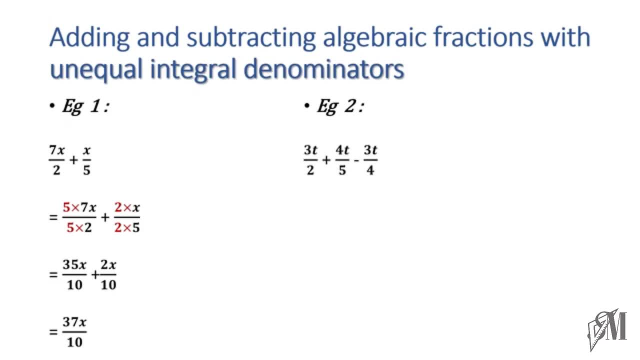 example: Here, once again you have three different denominators. Now again you have to equate the denominators 2,, 5 and 4.. If you think carefully, the least common multiple of 2,, 5 and 4 is 20.. 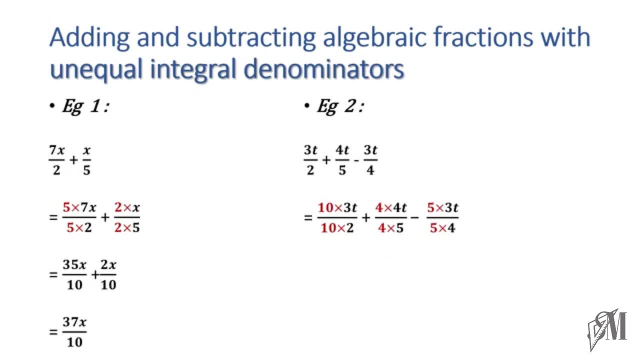 So, to equate all the three denominators to 20, we multiply the first fraction by 10, second fraction by 4 and the third fraction by 5, and then you will get everything over 20.. So once when you do the simplification, 30 plus 16t is 46t minus 15t will be 31t over 20.. Moving on to the third example, 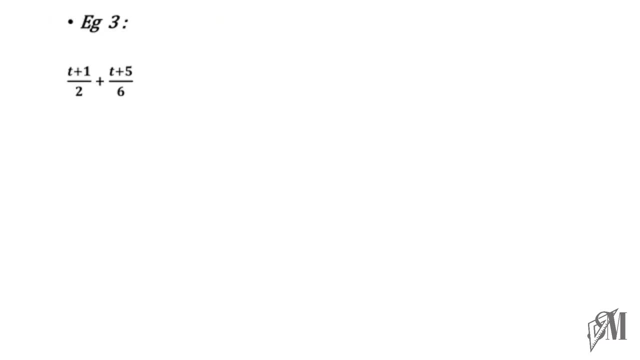 under this topic. that is here now t plus 1 over 2, plus t plus 5 over 6.. Now the- these are the numerators- are algebraic expressions, So to equate the denominators, you know, 2 can be multiplied by 3 and converted to 6.. So we. 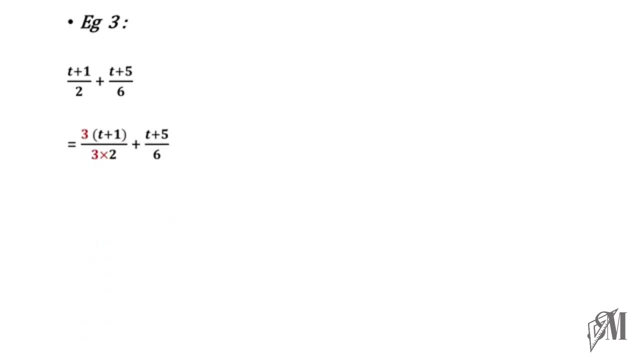 multiply the first fraction by 3 and remember if when you multiply an expression by any term, you have to bracket it and remove the brackets, otherwise you will do mistakes. So here I have put a bracket for t plus 1 in order to multiply by 3.. I hope you can remember how to. 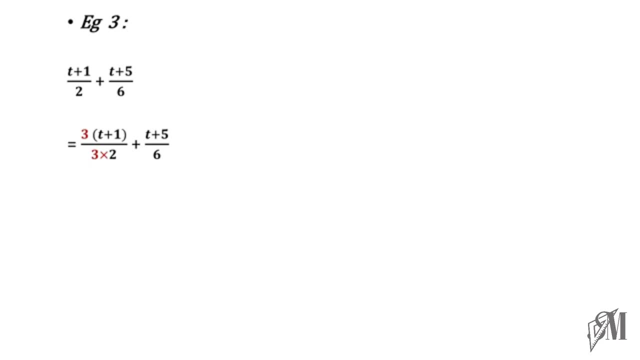 remove brackets and do the simplification here: 3 into t plus 3 into 1 will give you 3t plus 3 and this the remaining fraction I have written as it is over 6, and once when you add you get 4t plus 8 over 6.. Moving on to the next example, 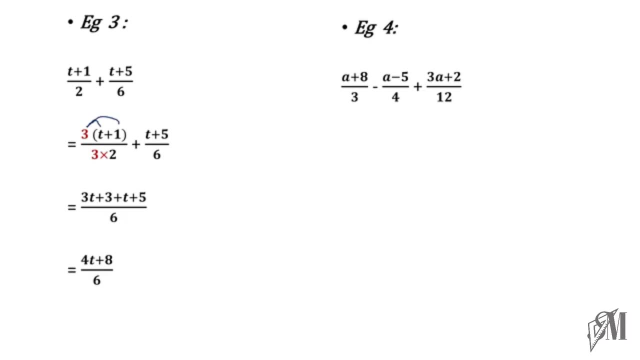 that is this. Now, here we have to equate all the denominators 3, 4 and 12. you know, 3 and 4 can be multiplied by certain numbers and converted it to 12.. So in order to do the multiplication, once again remember, we have to put brackets like this. Now, here you can see once when you remove the 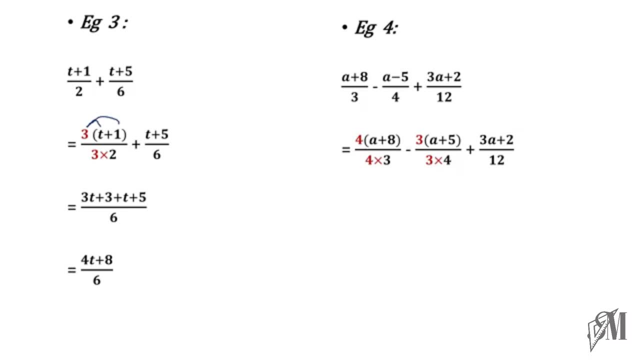 bracket 4 into a will be 4a, plus 4 into 8 will be 32 and minus 4 into 8 will be 32.. So this is the minus 3 into a is minus 3a and minus 3. I hope you can see why minus this. there is a minus sign here. 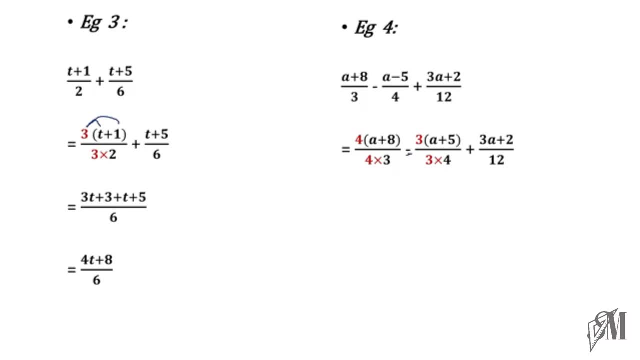 minus 3 into 5 will be minus 15, and so on. once when you do the simplification here, you will get it like this: Now you can see there is a minus 3a here. this minus 3a can be cancelled with plus 3a. 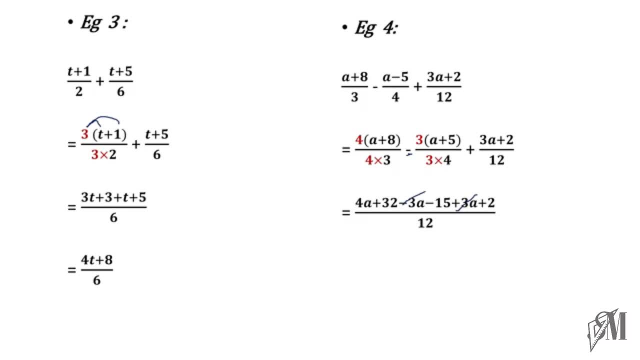 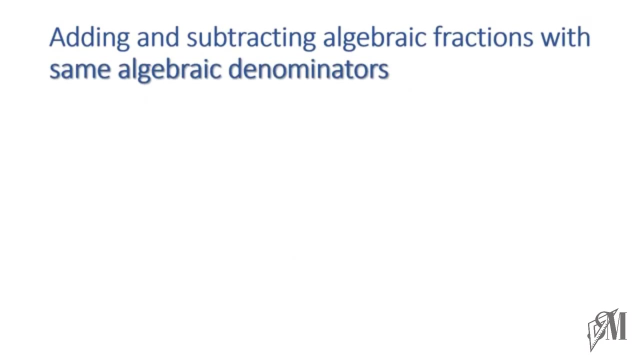 now 4a can be written as it is 32 minus 15 plus 2. Will be 19. so 4a plus 19 over 12 will be the final answer. Moving on to the next topic: adding and subtracting algebraic fractions with same algebraic denominators. Now here the denominator. 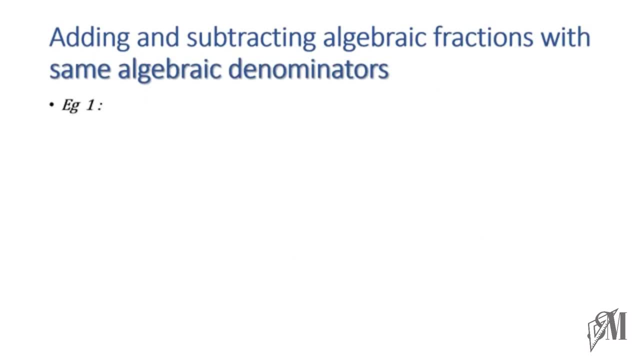 is algebraic. Now look at this example. both the denominators are 9y. very simple. you add the numerator 7 plus 6, that is 13 over 9y. Moving on to the next example: here, once again, all the denominators are 5 and 12 will be 19. so 4a plus 19 over 12 will be the final answer. Moving on to the 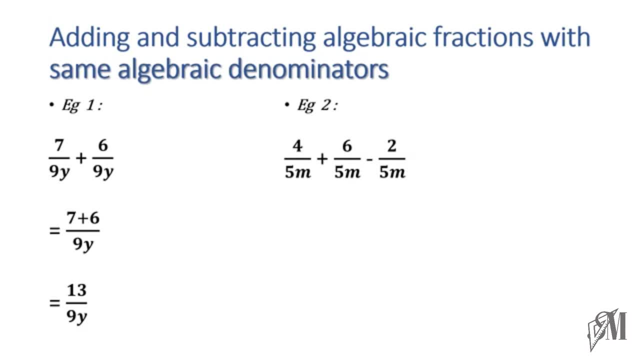 next example- here, once again, all the denominators are 5 and 12- will be the final answer. Moving on to the next example, here, once again, all the so 4 plus 6 is 10 minus 2 will be 8 over 5m. So 4 plus 6 is 10 minus 2 will be 8 over 5m. 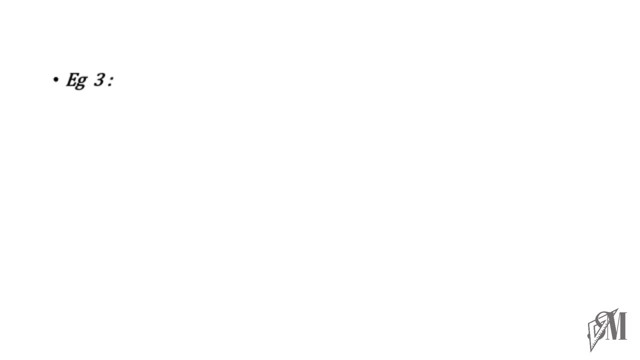 Then the fourth, third example here. now you have some algebraic expression and algebraic terms in the numerator, but still no problem, you can do. the same method of simplification is followed. t plus 60 will be 70 minus 3 over 4u is the final answer. Fourth example: 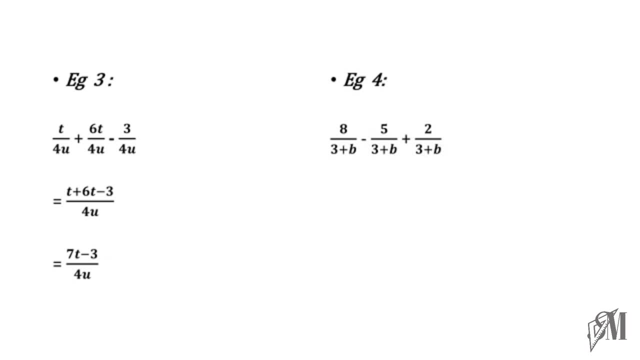 here the denominator is an algebraic expression, yet no problem, you keep it as it is and simplify the numerators. no, nothing to do with the denominators in this case, because all, all are equal to one another. so 8 minus 5 plus 2 is 5 over 3 plus b. right, this is very, very simple if the 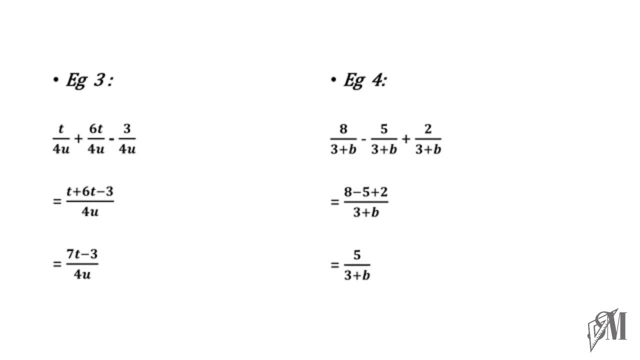 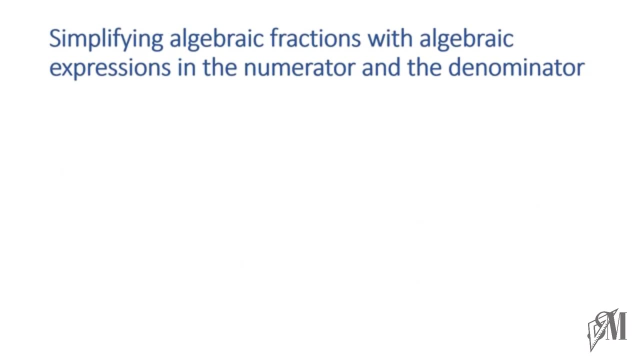 denominators are equal. the simplification is very easy. only if the denominators are not equal. we have to think a little Now here, simplifying algebraic fractions with algebraic expressions in the numerator and the denominator, both. now what to do, we'll see. look at this first example here, in both up and down you. 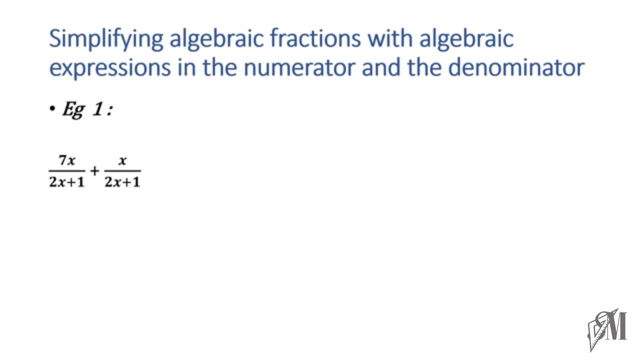 have algebraic expressions and symbols, so 7, but here in this case 2x plus 1 is the common denominator. therefore it's not a big deal. we can just add 7x plus x, that is 8x over 2x plus 1.. 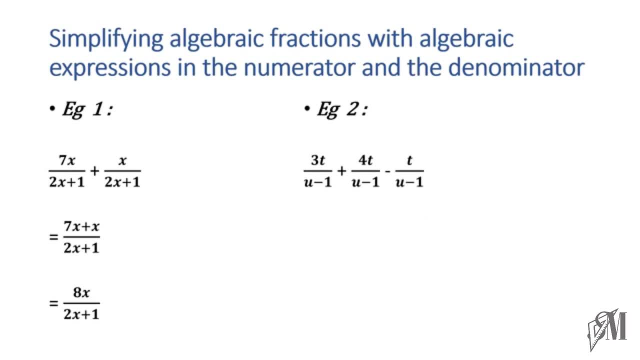 The next example. now, once again, here, the denominator is same- u minus 1- and the numerators must be simplified: 3t plus 40 is 70 minus t is 60 over u minus 1.. Now going on to the next example. now look here. 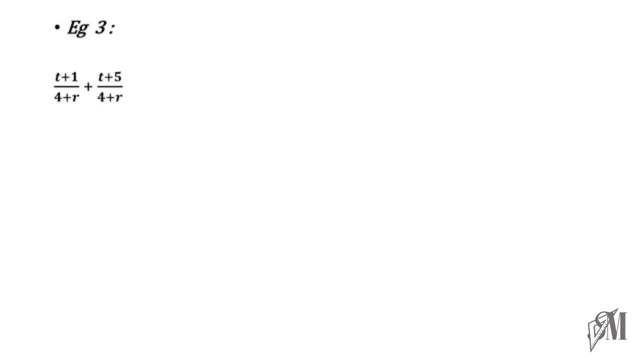 t plus 1 over 4 plus rt plus 5 over 4 plus r. the denominator is 0, so at all 4 plus r. that means 3t plus 5 over 4 plus 1.. is same, so we write the rest of the numerators in one line like this, and then we do the. 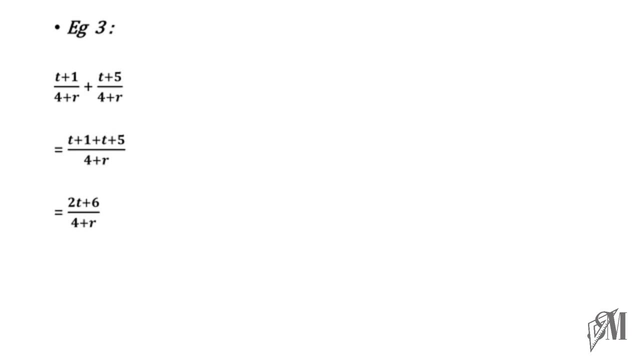 simplification: t plus t is 2t, 1 plus 5 is 6, so 2t plus 6 over 4r is the answer there. the fourth example: fine, now here all the denominators are equal to a plus 5, so nothing to do with the. 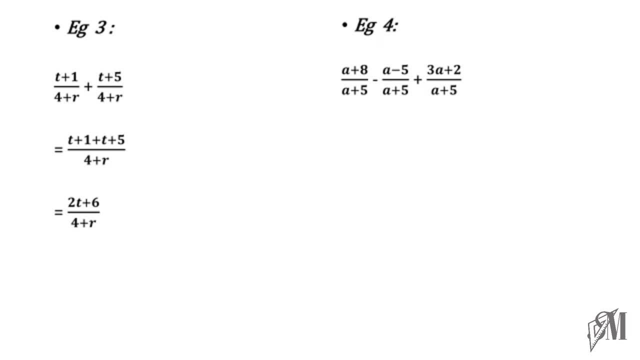 denominators and, in this case, numerators, must be carefully simplified because there is a minus sign or there is a subtraction. so, as i said before, you have to put a bracket like this before simplifying, and then you have to make sure to remove the bracket minus into a and minus into. 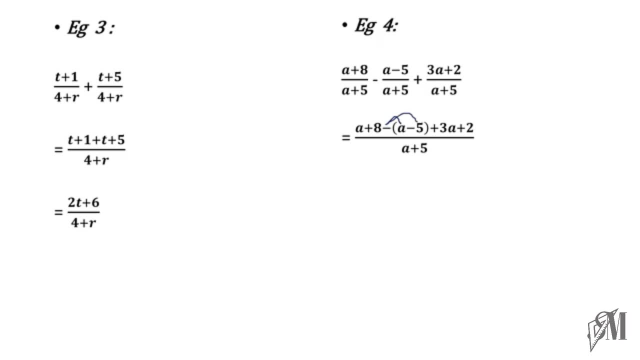 minus 5. so once when you do that simplification, you get a plus 8 minus a minus into minus 5 is plus 5 plus 3a plus 2. so once when you do this, then you can again see this. a can be cancelled. 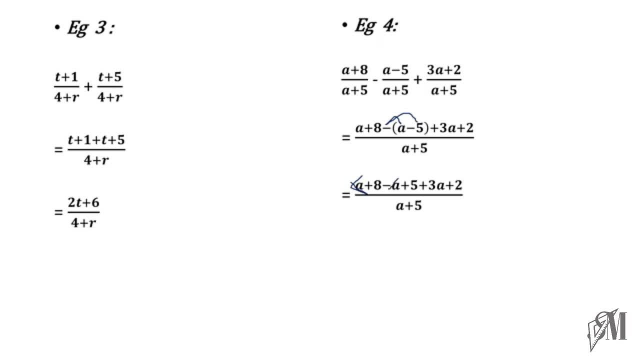 with this minus sign. so you have to put a bracket like this before simplifying, and then you have to. then you get 3a plus 15 over a plus 5. now, once again, 3a plus 15. you can see 3 can be taken out. 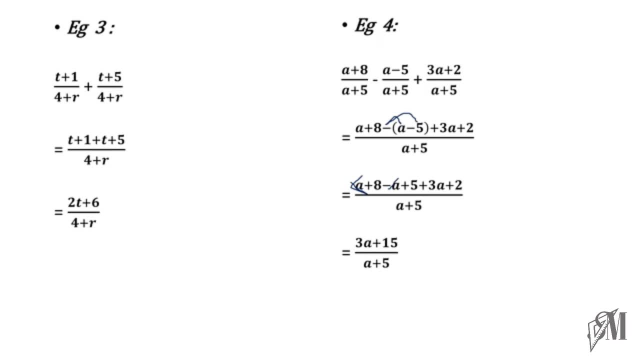 because 3 is common to both 3a and 15, so you can take 3 out of a bracket like this and then what is remaining- a plus 5- will remain inside. now, in this case, this a plus 5 and this a plus 5 can be.